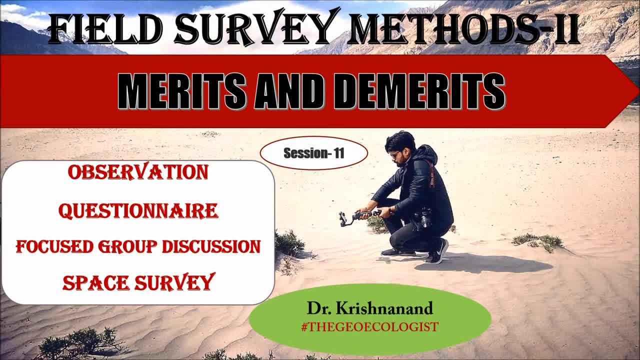 Hello everyone, welcome to the Geoecologist. In session 11, we are going to discuss about field survey methods, part 2.. So in the earlier part we discussed about the various advantages, disadvantages and various functions and structure of the field survey methods. So in session 11,, 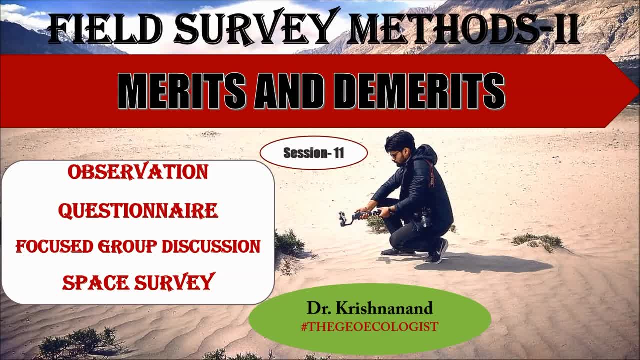 we are going to discuss about four specific field survey methods, That is, observation, questionnaire method, focus group discussion and space survey. Alright, so we are going to discuss this, but before that we will be talking about the requirement of the methods, why and. 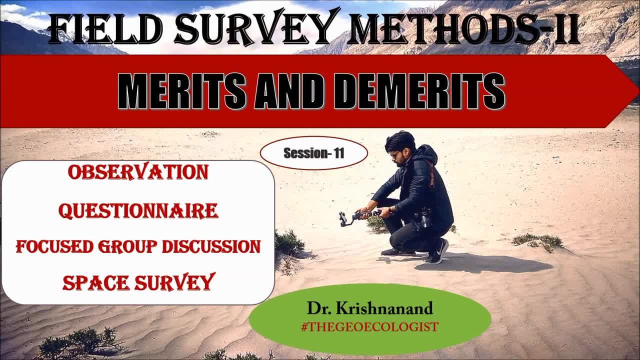 which method is to be selected and its various merits and demerits, That is, the advantages and the disadvantages. So please focus upon all the things that are going to be discussed today in this observation questionnaire, focus group discussion and space survey, along with its 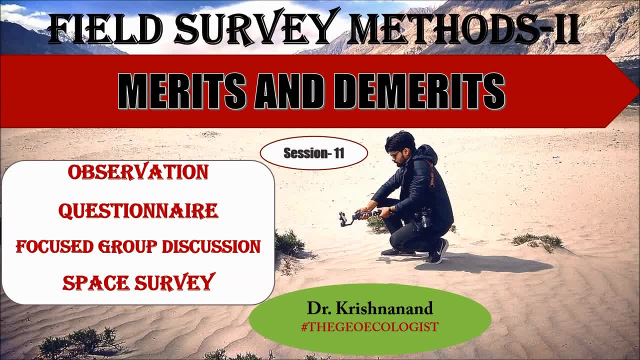 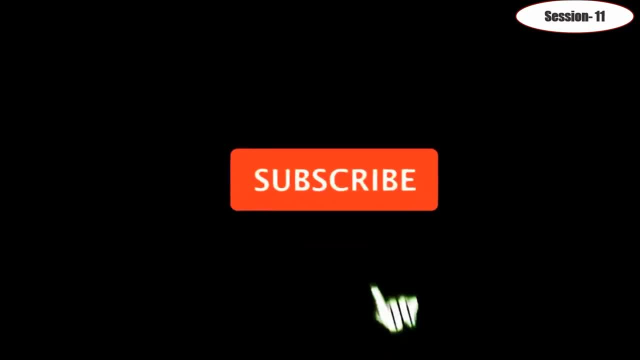 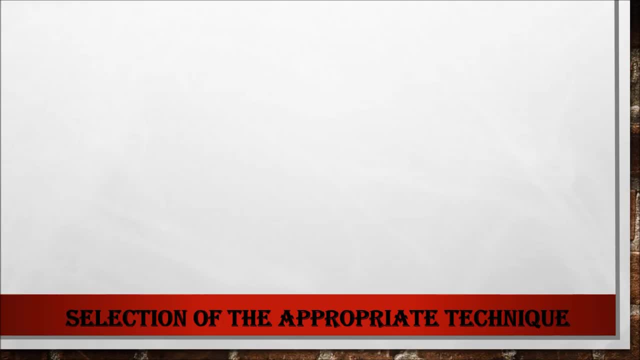 advantages and disadvantages, So that you can utilize it for your fieldwork whenever you want to carry it, Alright. so, before we go further, please like and subscribe to our channel and please press the bell icon for the updates. Now let's go ahead and see the selection of appropriate technique. So what is the key? 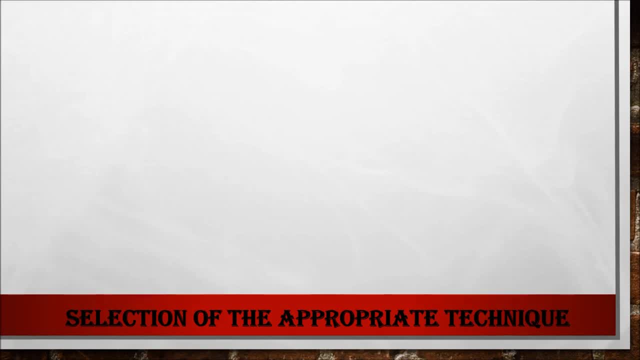 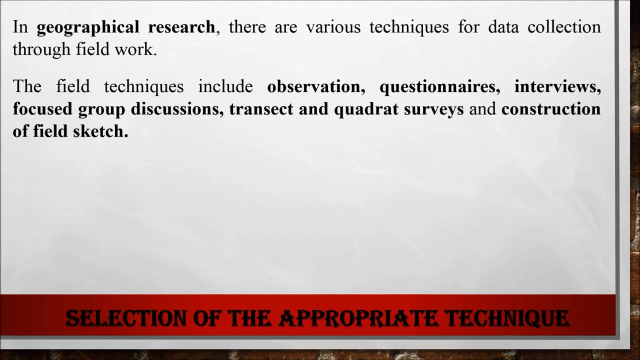 behind selection of appropriate technique. How do we know that Right? so let's look at that. So in geographical research there are various techniques for data collection through fieldwork. The field techniques include observation, questionnaires, interviews, focus group discussions, transect and quadrate surveys and construction. 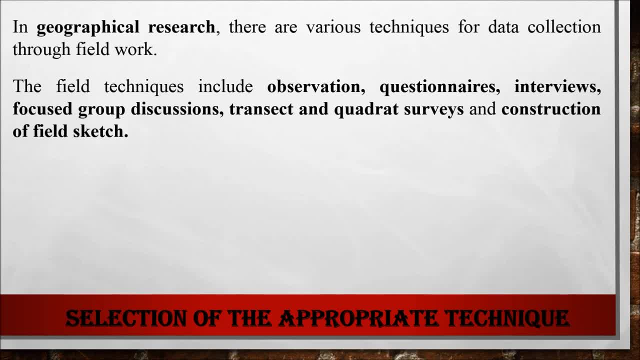 of field sketches. So these are the various techniques that we use in the field for data collection. So all these techniques have to be appropriately selected based on objectives of the study. So remember, the key lies in your objective of the study, not in the technique. 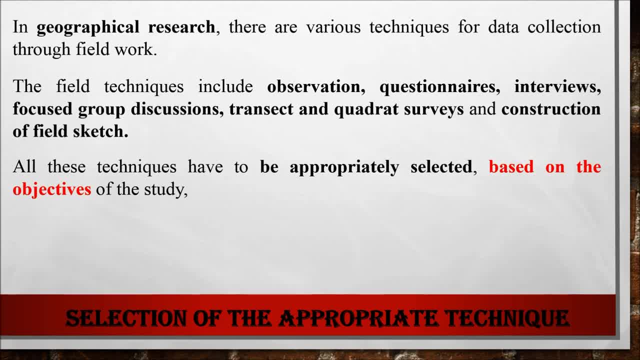 itself. So, whatever be the objective according to that, we need to understand that what will be our technique that we are going to use for data collection for the purpose of the study- So it can be geographical, socio-economic and cultural context that we're going to study, and resources. 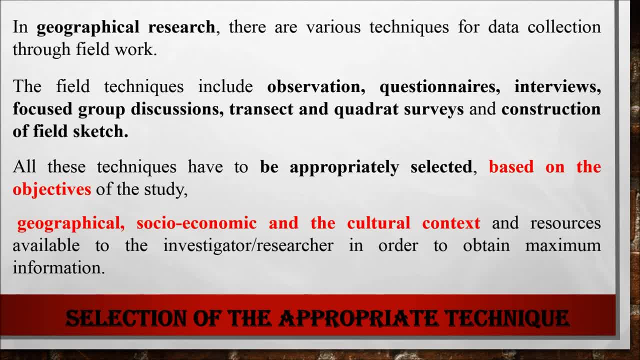 available to the investigator or researcher in order to obtain maximum information. That is the whole idea behind this selection of appropriate techniques. So the first thing that I wanted to pitch is: the appropriate technique is based on the objective of the study and the context of the study. If we are very clear about our objectives and the context of the 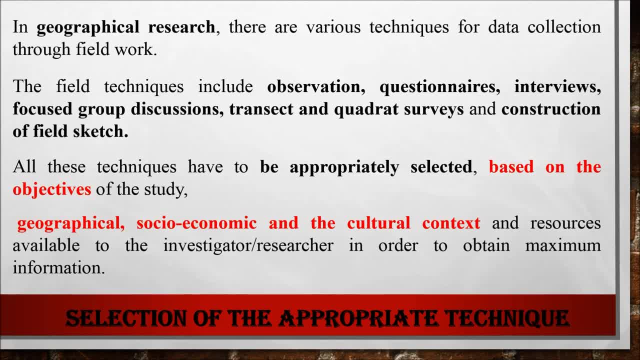 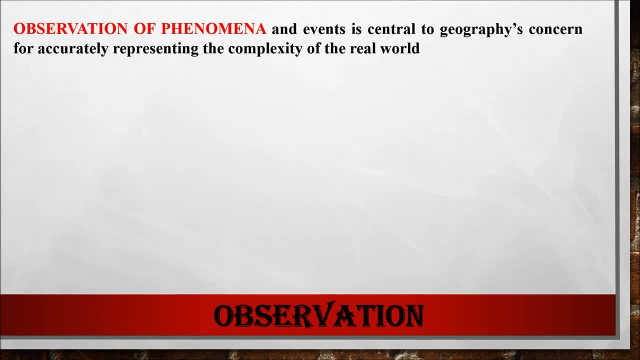 study. then we can select the appropriate technique. So that is the key. Now let's look at the first way that we look at a particular phenomena in the field. So first technique that we learn is observation. So observation of phenomena and events is central to geography, geography- 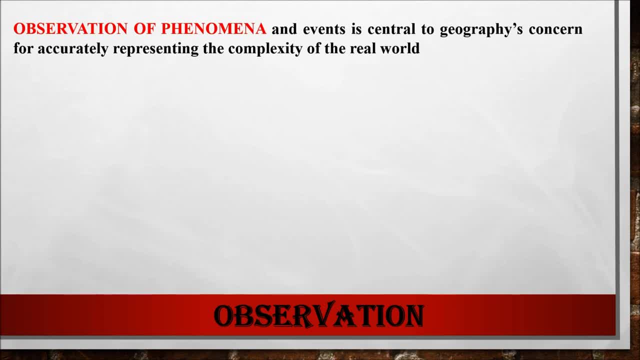 and many other social sciences. main theme of data collection- right because it's the main concern- is accurately representing the complexity of real world. so when they, when we go to the field, we see that real world is not simple: it has, it may have complexity and the data also may have. 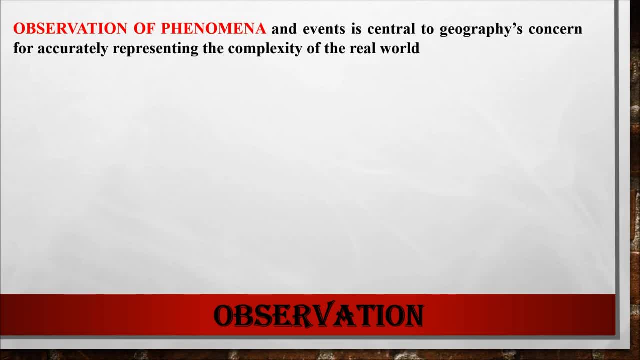 complexity when we want to collect it. so observation is one thing that is very much central to geography's research method, right? so observation can be simply defined as the way of gathering data by observing behaviors, events or noting physical characteristics in their natural setting. so this is the simplest way observation can be understood. so to observe means to observe behavior of people. 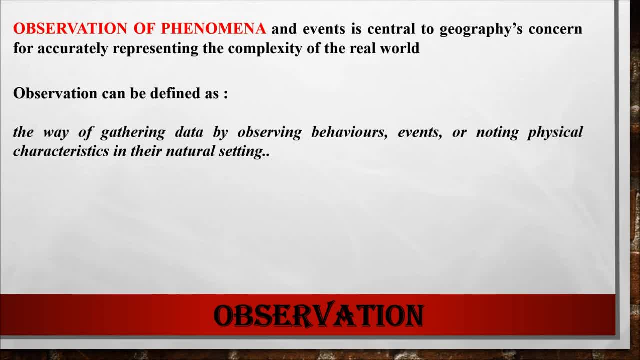 or maybe, for that matter, animals, flora, fauna as well, also, depending upon the study, the events that we are studying, the events that we are talking right, and also the physical characteristics in their natural setting, in their in situation, in situ, right. so that is what observation basically means. now, observation is of two types. many a times people don't understand. 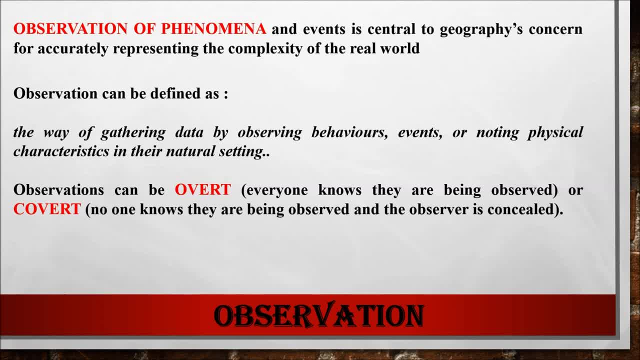 what is the difference? it is overt and covert. so many a times when we talk about overt and covert, people don't understand how to delineate or distinguish one from other. so overt operation is: everyone knows that you are being observed. so if you go to the field and sit someplace and 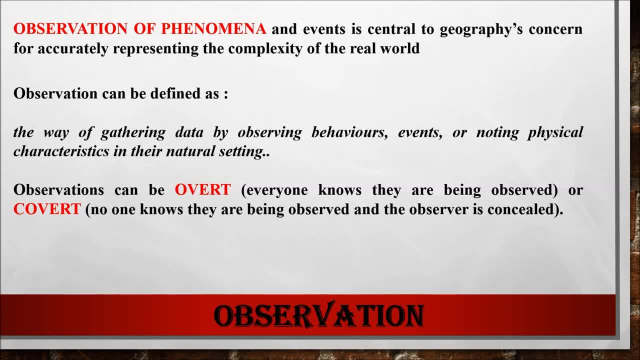 you're observing people. what happens, people understand. okay, he has come to study us, he has come to observe us. that is overt. but when you go secretly, no one knows that you're observing certain behavior or certain event in the field. that is covert, so no one knows they are being. 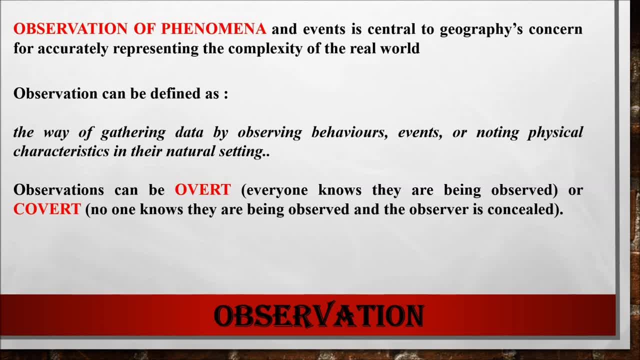 observed. so observations are of two kinds. now depends on our contextualization of study- again, objective of a study, that what kind of observation do we want: overt operation, overt observation or covert observation. so that is very much common, that what kind of observation will depend upon what is the main objective of the study, right? so now let's look at further. 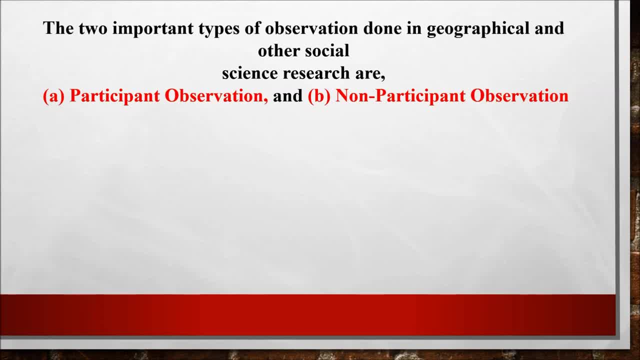 the major types of observation in the field or the science: researcher, participant observation and non participant observation. all right, as the word itself says, participant it means we as researchers have to participate in the phenomena itself, in the event, in the locality, with the people. and if we are not participating then it is non participant observation. 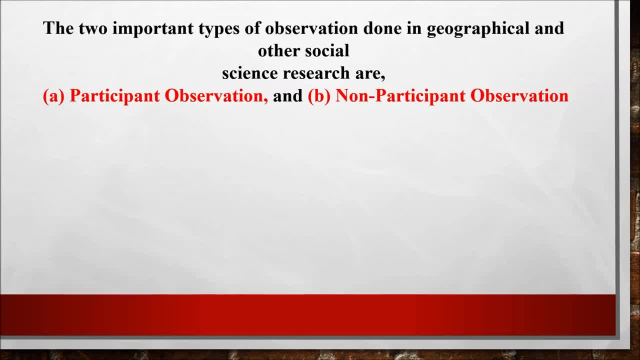 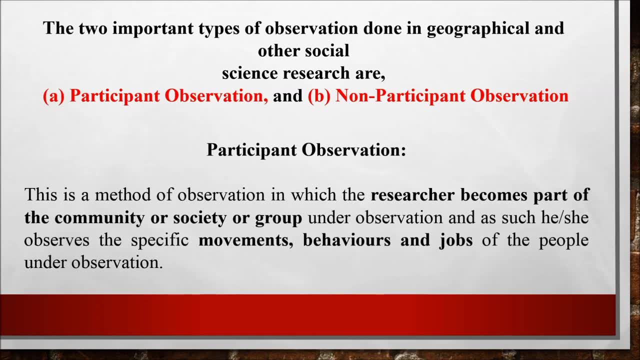 if you're participating in the activities, with the people, with our respondents, then it is participant observation. so now let's look at the concept. so participant observation is a method of observation in which researcher becomes part of the community, as I said. so we have to become part of the 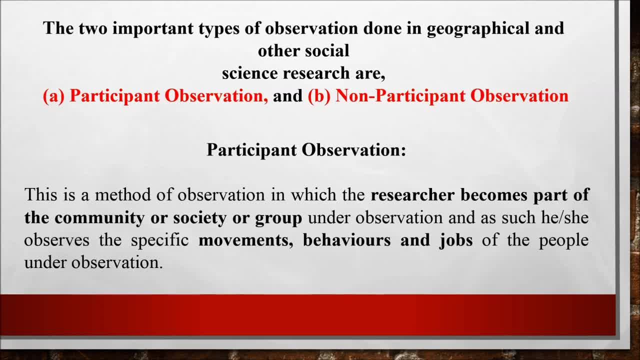 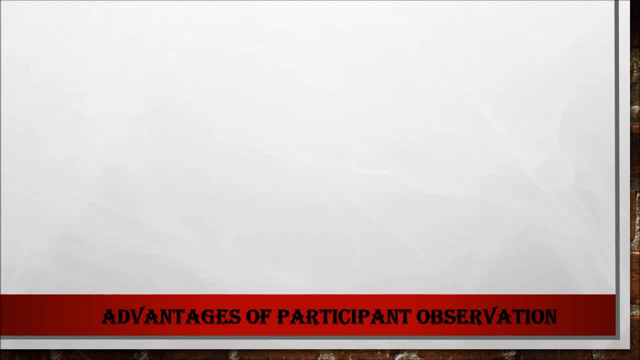 group, right. so specific movement behavior, job of the people, these things are being observed while in participant observation. so what are its advantages? let's look at that observation of natural behavior. when you're participating with people, you're making a close contact, right? so what happens? you're studying them in their natural behavior. suppose you're going. 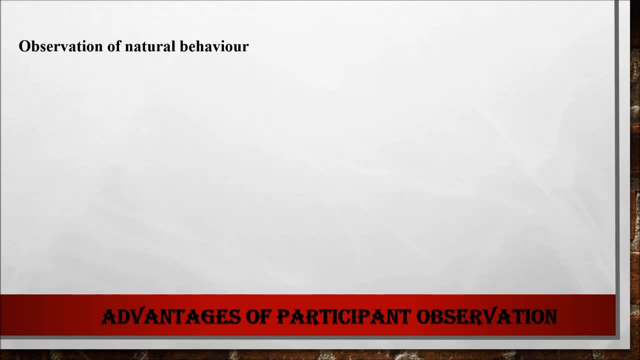 to the field where maybe a person is plowing or planting something. so you start planting with him. he will not behave differently with you, will think that you are his, you know well wisher and you have come to help him. so if you bring a wrap-up factor there, so natural behavior. 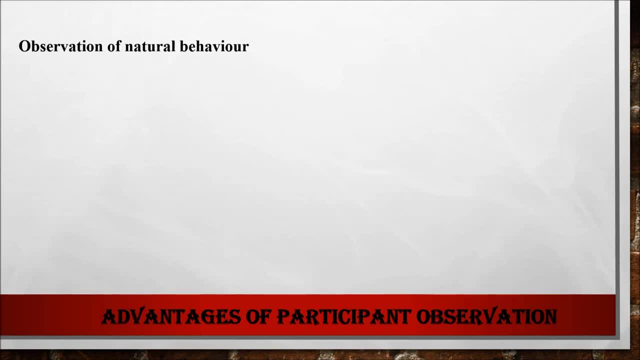 of a person can be observed. a agriculturist may behave differently if you start asking questions putting a paper in your hand. so observation is one thing that will give you natural behavior study right then, proximity with the respondent. as I said, proximity is very much important. wrapper building, as I said. ethics of field work: we have already. 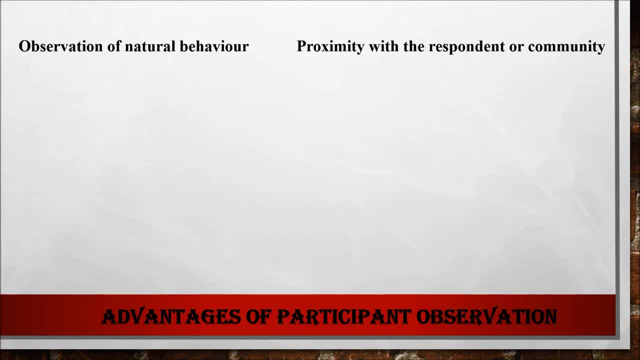 studied. so wrapper building is dependent upon this method of observation. if you are in participant manner, right then, identifying the real character of the place. so if you want to identify the real character of people place, their interaction, this is the method. observation in a participant form, right then better understanding. obviously it will give us far better understanding than 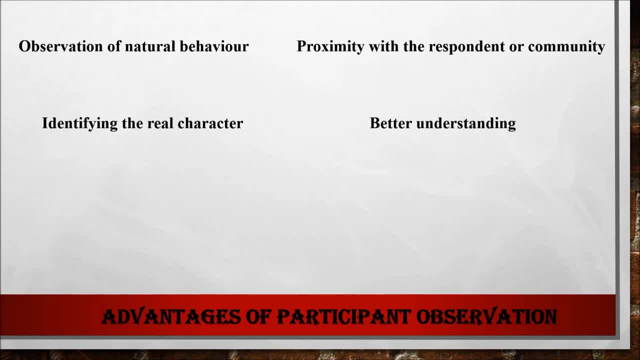 observing from a distant right, then participation observations. you know it provides opportunities to learn more about phenomena, geographical location and event. so this is one ahead part that it also gives us opportunity to study more, not remain fixed to our objectives. so it will give us an opportunity to learn more and more, even if it is not part of our objective. 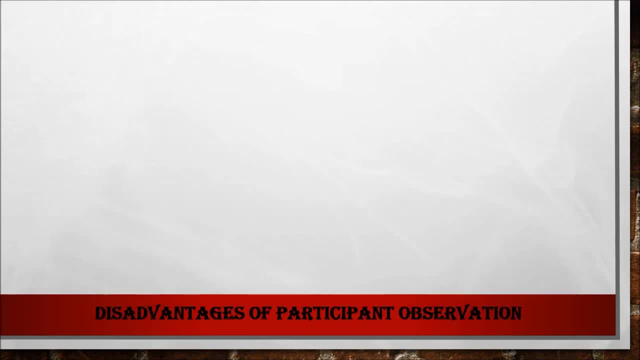 but there are certain disadvantages also of participant observation. first is lack of objectivity. this happens because when we are in proximity with people, we tend to lose certain things that we are not aware of, and we tend to lose certain things that we are not aware of, and we tend to lose certain things that we are not aware of, and we tend to lose certain. 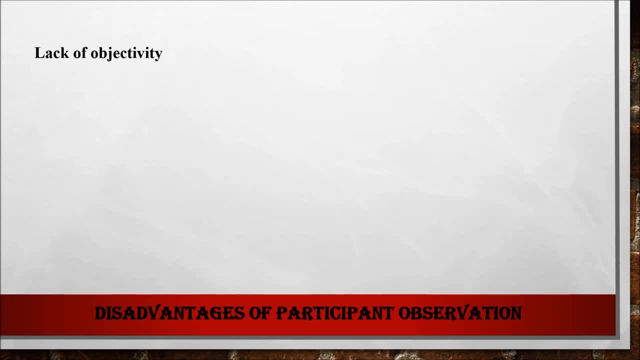 objectivity. so what happens? things become very subjective in nature, right, because we are now too much involved in the situation or in the events. so often close association brings biased interpretation. suppose if I become friends with a person, with family, the response group in the feel so I will be biased towards him. may be because of certain opinion. 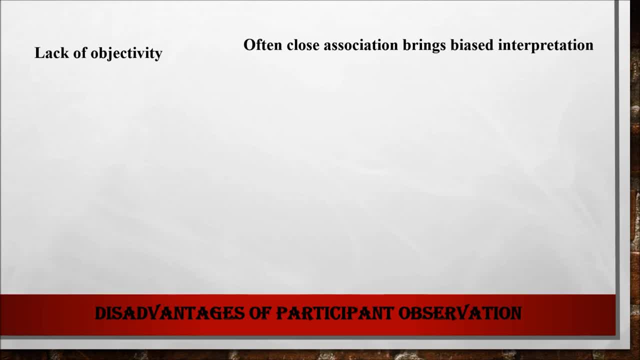 isn t it? so this may come into the picture as a limitation. then again, range of experiences is very limited, because now you are fixed with the particular participant, isn t it so happens the range of experience is limited, then there is a chance that we miss out on many. 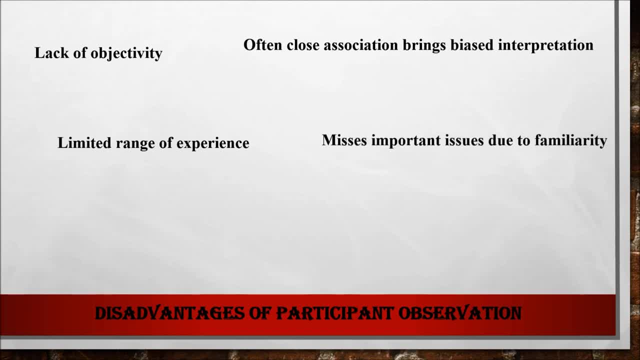 opportunity of familiarity, all right, with the phenomena, with the surroundings, because we are too focused on just a single part. then there is a limit of participant observation, right? so what happens? participant observation has limits in a way that you cannot intrude too much into the society, that is. you know, it's always a problem that you're an outsider to the society. so if you 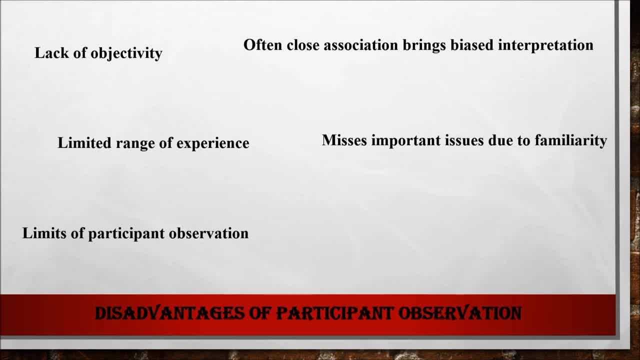 start too much of you know, poking your nose in somebody's job, then it will make it difficult. so there is a limitation in that participation. right, and then do not get involved in groupism. this is another fallback that maybe there are certain groups of people in your society. 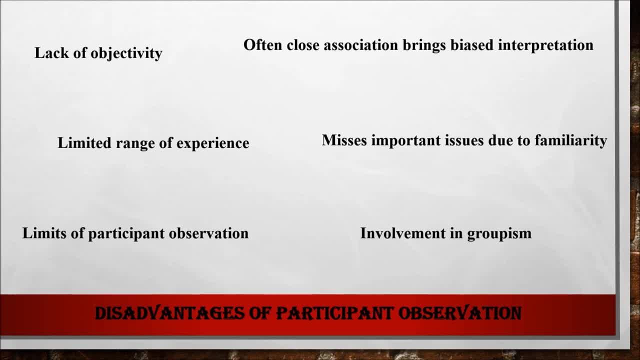 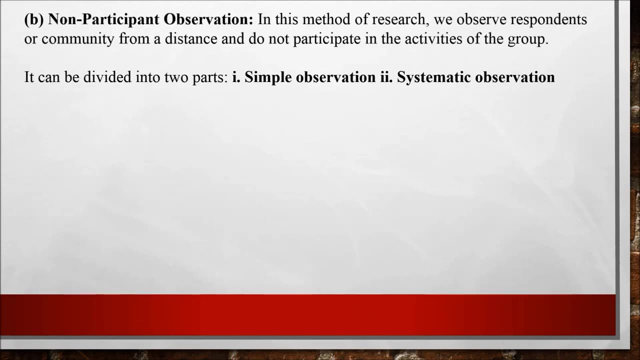 one doesn't like the other, then you fall into certain group because of your participation. then there is a disadvantage, so this may happen. so these are the disadvantages of participation. observation. now, non-participant, as we know, non-participant is: we directly do not participate, but from a distance we observe it right. so it is simple observation and systematic observation. 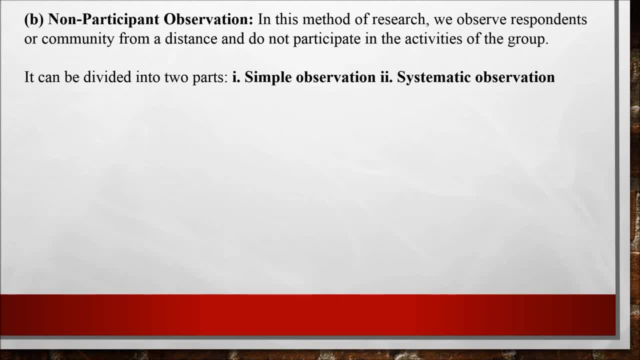 these are the two types of non-participant observation. simple is: researcher keeps himself at a distance from the group under study and observes records, collects data, but there is no usage of data collection tool, for example, no schedule, no questionnaire. these things are not involved, simply looking, sitting at a place and just observing from a distance. 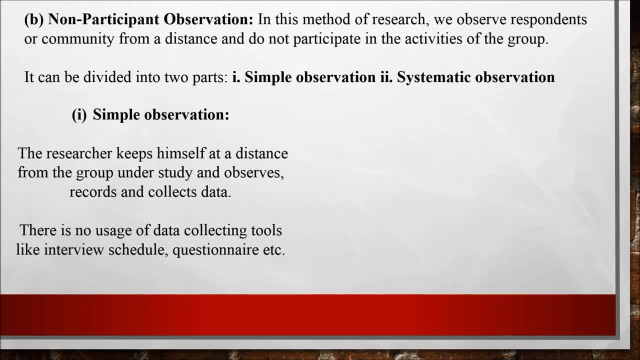 right, that is simple observation, but systematic observation. the researcher adopts a procedure by framing questionnaires or schedule, because it can be carried out in a common social condition in the field. so many times if you sit at a tea stall or a junction where people come and gather, 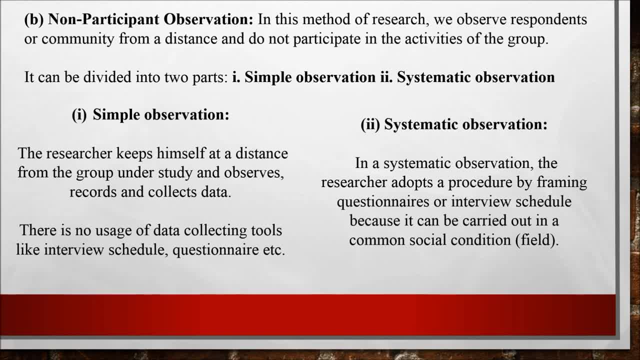 so you can also ask people questions and you can, you know, observe how they behave when you ask them questions. so this is something, a systematic observation, but from a distance you can observe, right, you don't need to get into their lifestyle, you can. you don't need to get into their shop and start selling items for them, you know, you don't need to. 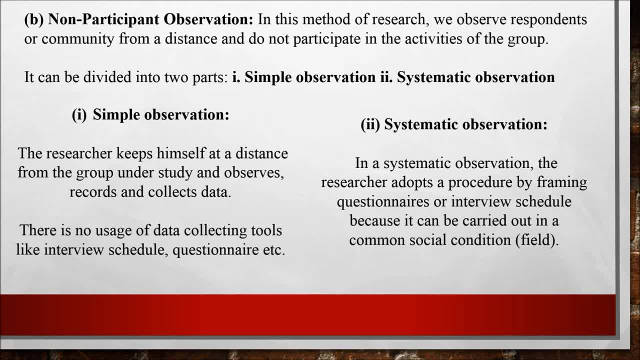 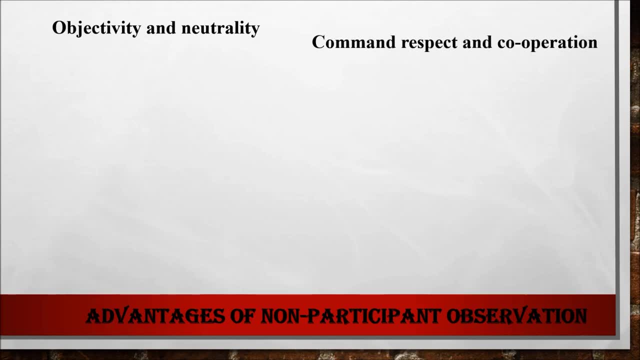 get into the agriculture fee and plantation stuff. that is when you're doing participation. but this is non-participant. all right now. advantages of non-participant. obviously, objectivity and neutrality will be maintained. that was not there. command, respect and cooperation. this is important that this will command you respect and cooperation as well at many times because being at a distance, 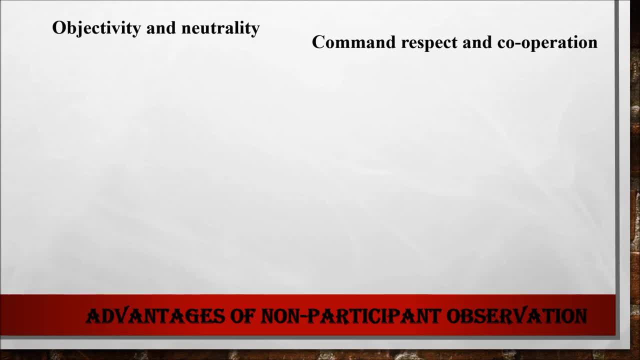 you can build a rapport with a person in which there is a certain mutual respect for each other. many times when a person starts to know you and know your initiatives, that is because of a selfish interest. they may fight with you. they may do not, you know, restrict themselves. so respect and 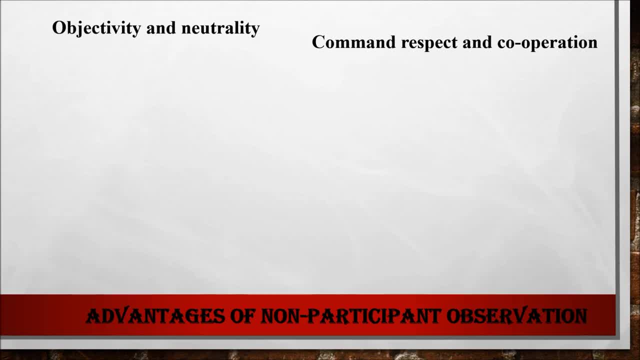 cooperation is expected. careful analysis is the best part that you can without participation. you can focus upon the complete phenomena in the picture and more compliance of respondent. so what you can- comply with the respondent in a more focused manner, that is very much important. and freedom from groupism, that is the best part. that in non-participant observation you do not. 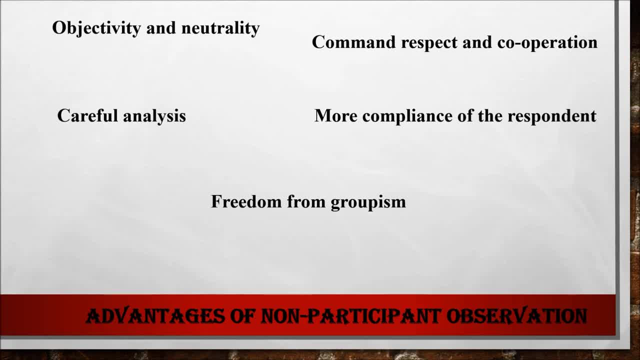 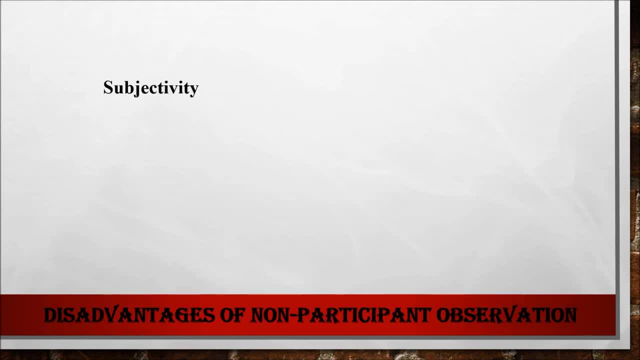 have to worry about any groupism because you are a neutral person observing from a distance. right, then we have disadvantages. so, again, subjectivity is involved. at many times, reliability of data can be a question because you are not observing it directly. you are from a distance, so you may interpret in a different manner. 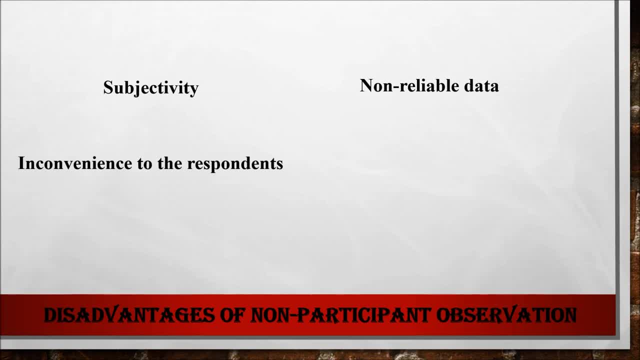 so this is a problem that we have to be careful in this regard. you may get involved in the observation of the data and the data is not being observed in a way that is in line with the participants observations right. so this is one of the disadvantages is another part, because when you are observing somebody and they get to know, it becomes 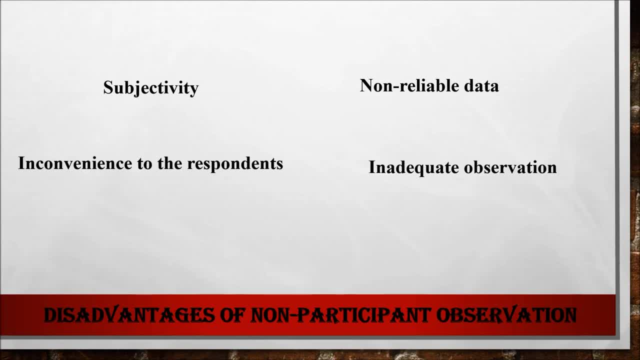 inconvenient for them many times that this person is coming every day and sitting here and looking at us working. you know so this is a problem, so it can create a suspicion. so inadequate observation is another part that you cannot maybe able to observe adequately unless you get involved. that was part in the participant observation. so these are the disadvantages. right now let's look at the next method. 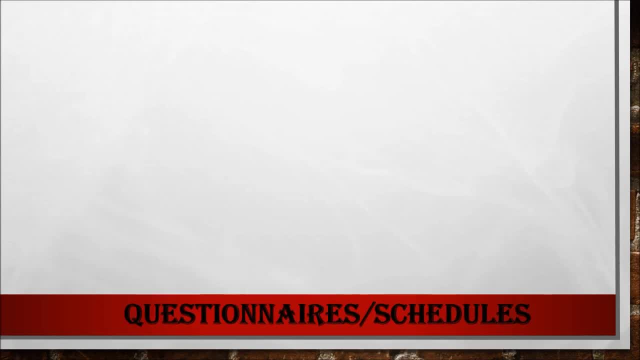 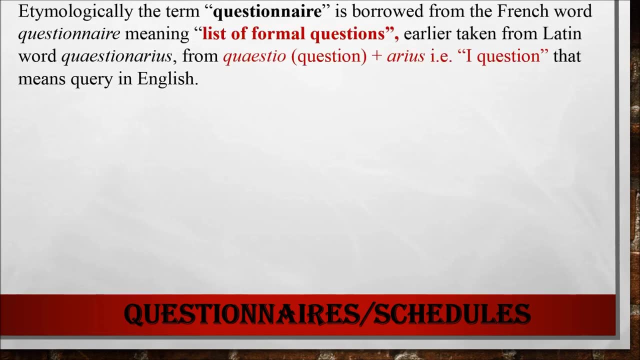 after observation. the next method is questionnaires or schedules. right, so first let's go. what is a questionnaire? so the word comes from French word that means list of formal questions. so, very interestingly, it means list of formal questions and it has been derived from French and then Latin as well, that is. 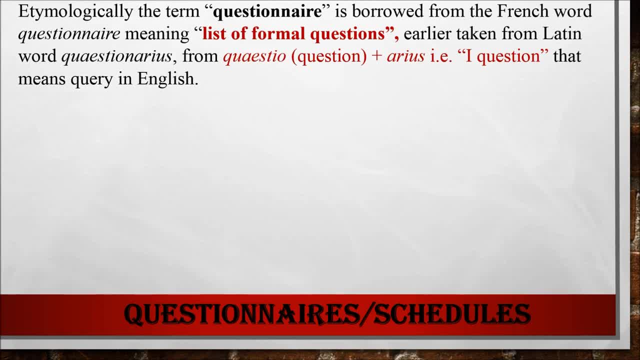 question. that is questions and arius is I question, so it basically means a person who is questioning this list of formal questions. that's how the questionnaire has come to the picture, right? so definition of a questionnaire: first idea is a set of questions for obtaining statistically useful or 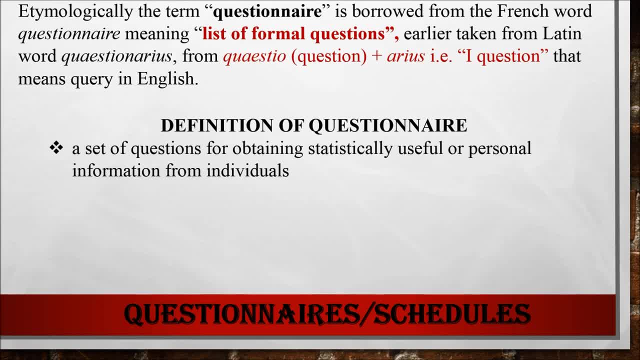 personal information from any respondent or individual. that is the first basic definition. it can also be understood as a written or printed questionnaire, often with spaces for answers. that is another part- then a survey made by use of questionnaire. this is a simplest definition. so these are the things that 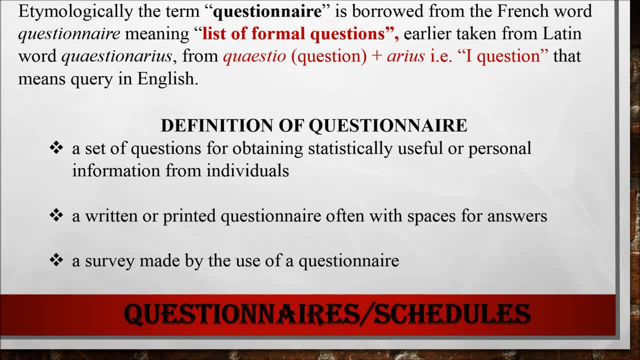 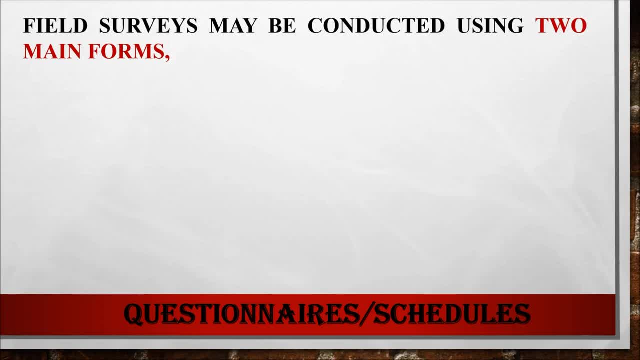 you need to understand what is a questionnaire, and next we go then questionnaires and schedules. so field surveys may be conducted using two main forms. first is by putting questions by an interviewer and answers recorded on an interview schedule which sets out the questions and provides room for the 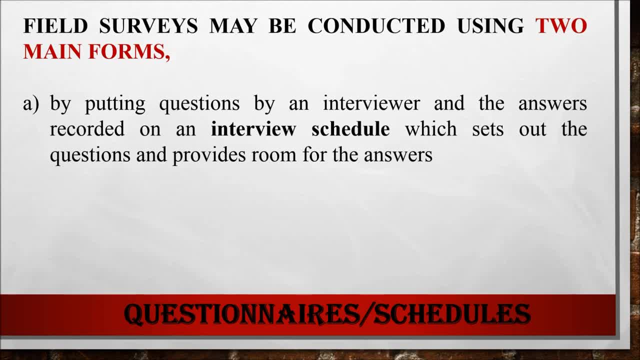 answers. so one is when, as a researcher, we ask questions and people respond and we write it or record it. that is schedule, okay, in which the person, the respondent, doesn't have to do it themselves. we are there to support and to record, to write their answers. right, that is a scheduling. then a questionnaire. 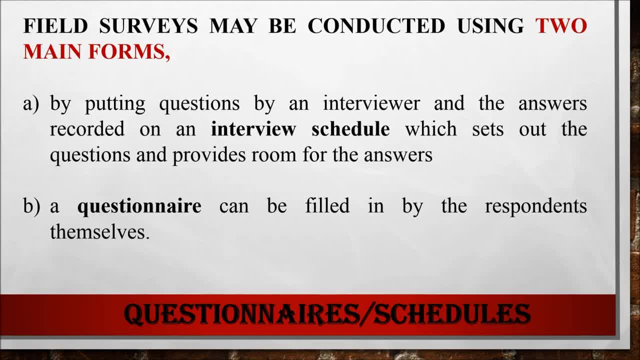 can be filled by the respondent. so remember there is a difference between questionnaire and a schedule. questionnaire is filled by the respondent, schedule is filled by the researcher. so that is the main difference and remember this difference. right then, types of questionnaires. so the first type that we 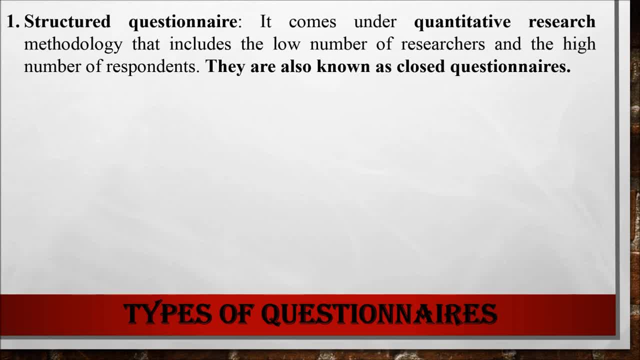 go on. the structure of the questionnaire is structured question. it is largely quantitative research methodology that includes structured. the name itself is that, so it has a proper format right, and then many times it has closed questionnaires involved in that. so what happens? the answers are fixed. the 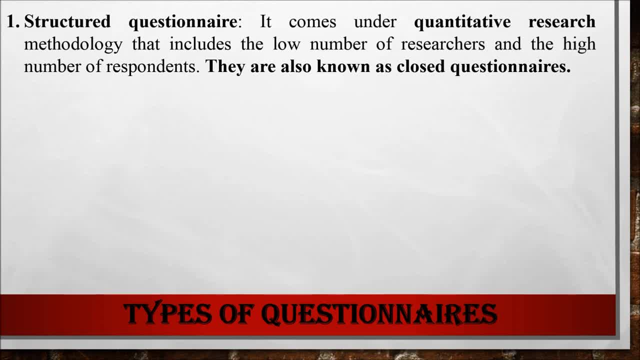 options of the questions as an answer are fixed. suppose I ask somebody what is your income? so I give the answers 10 to 15,000, 50 to 20,000, 20 to 30,000. so I am giving an answer. it means I have fixed it. so if somebody is not falling in the 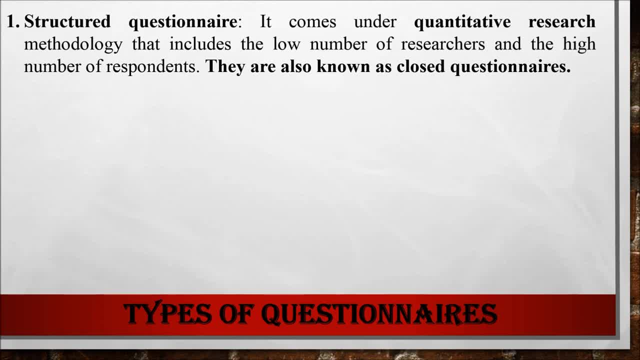 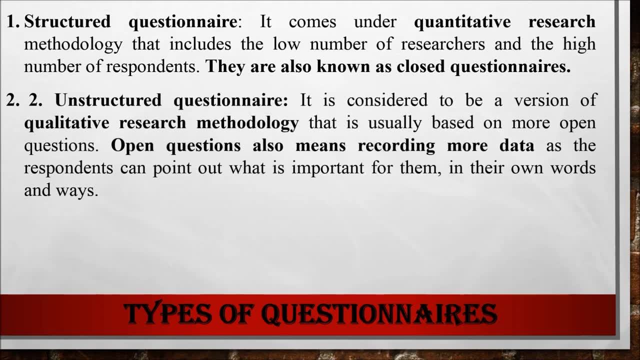 group, then it will be a problem in this kind of questionnaire as well. so unstructured questionnaire is the next step. second part: so it is considered the qualitative research methodology question. so these have open questions like, for example, what is your experience in this business all about? so then people will respond and you can write it. 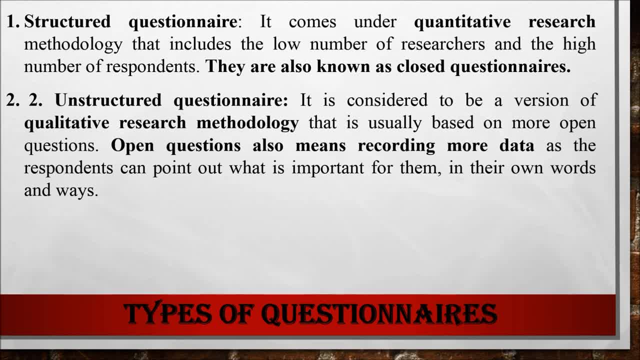 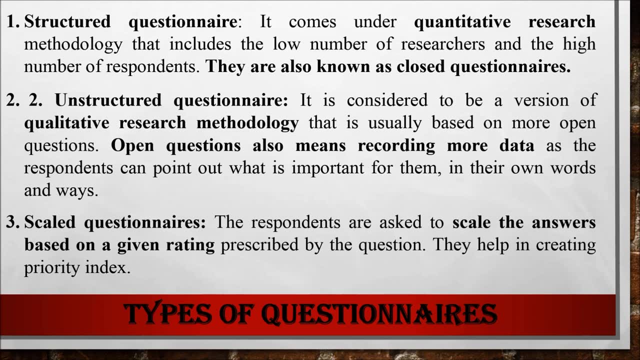 isn't it? so it's not. it doesn't have a fixed answer, so it's not closed, it's open end. and then scaled questionnaires. so then scaling is involved, means the rating is involved, suppose I say that rate the maximum to minimum or minimum to maximum advent of tourists in this particular season. what is the most? 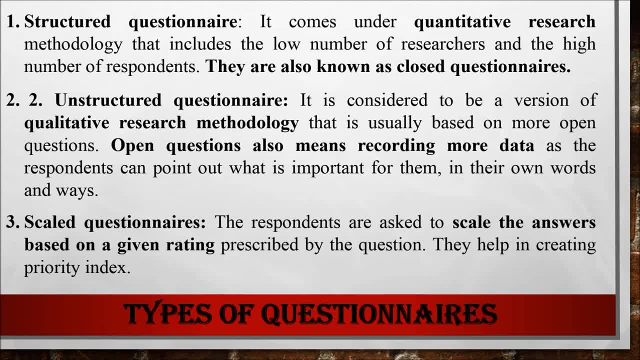 selling item in your shop. if I'm going for a market survey, so I ask them rank these five fruits in the nature of their sale per season, so which is the most selling, which is the least selling. so these can be a scaling right, so that becomes another important. so structured, unstructured and scale questionnaires. 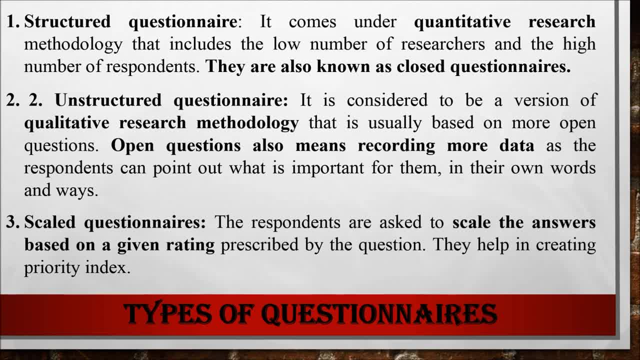 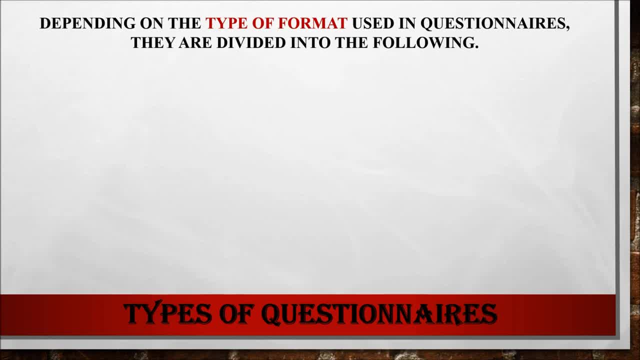 depending upon our, again, objectives of history. so these are certain types. then we have more types. so this is depending upon the formatting used in questionnaires, divided into following segments. first is the open-ended questionnaires. as i have said, they are open because they have types of questions that allow respondents to express them freely. 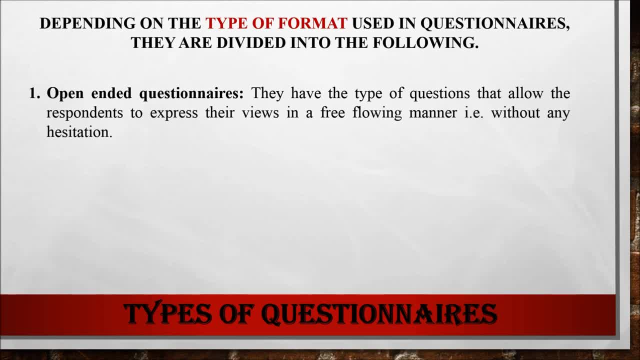 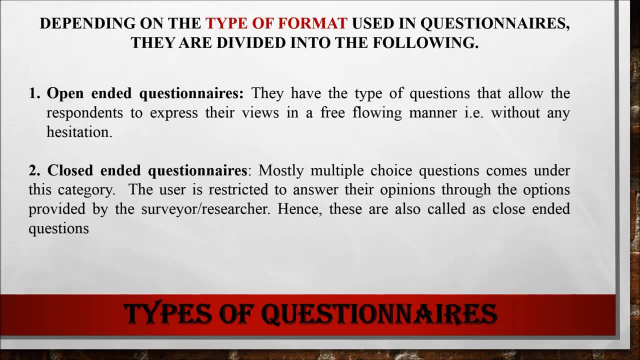 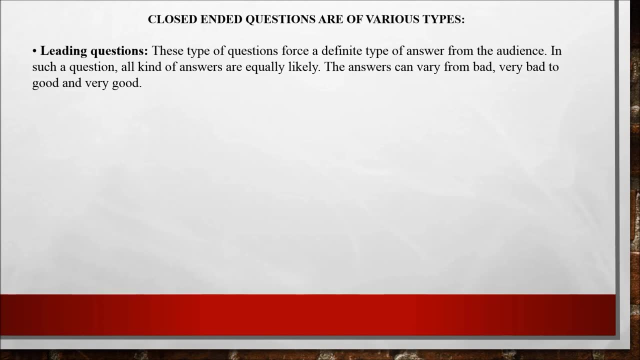 that's why it is open-ended, closed-ended. then they have multiple choice questions which are fixed in categories. hence what happens: user is restricted to answer from the options that has been provided now. closed-ended questionnaires have certain types of questions, so these are very much important questions. the first is called leading question, so leading question is a type. 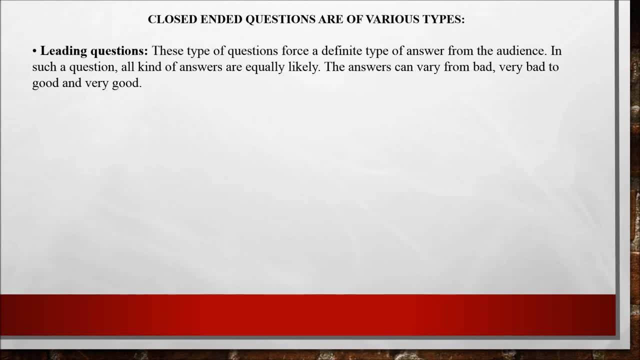 of question that forces an individual for a particular kind of answers that you are demanding because you are leading him to answer right then. importance question, for example, the respondents are asked to take rating for a certain type of issue on scale one to five. suppose i ask that. 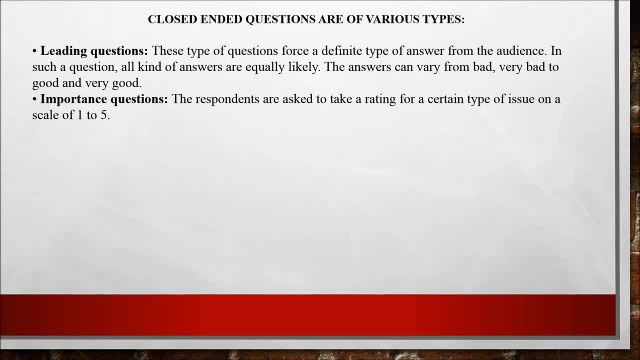 do you think that there is a decline in biodiversity because of climate change? if you think, then what do you scale it so one to five? so if you are saying five, it means you have five, five, the same viewpoint, as it is mostly affected, right? so this is importance question. then we have 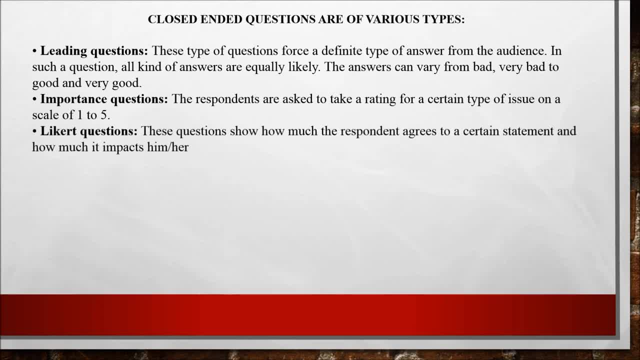 liquored scale, that is, questions, show how much the respondent agrees the degree of agreement to a particular statement. so if i make a statement that because of climate change there is a biodiversity loss, do you agree to it in one? what degrees? so, strongly agree, moderately agree, disagree. 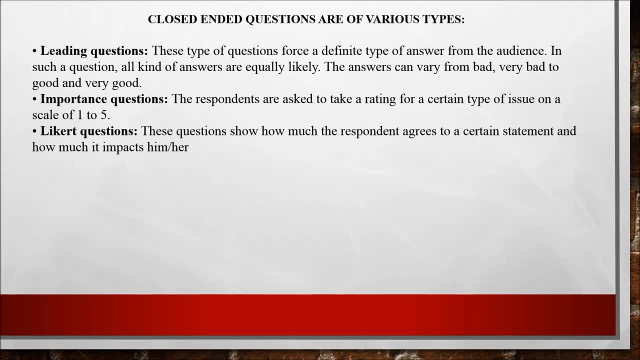 or no answers. so these kind of agreement questions in a statement form forms the liquor questions. right then dichotomous questions. these questions ask the respondents only yes or no. that's why it is dichotomy, hence it makes difficult to analyze beyond yes or no. remember so very few. 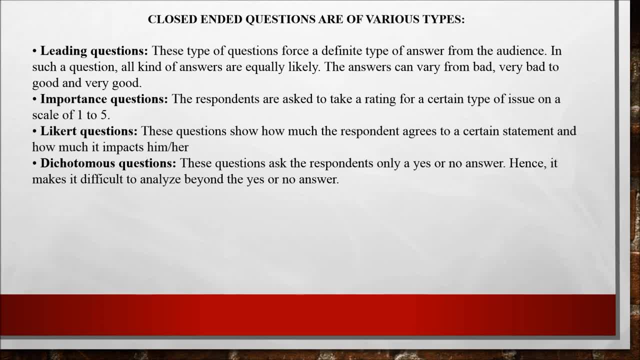 questions can be asked in dichotomous ways and be very careful when you are asking a yes or no question. bipolar question: such questions have answers that are extreme in nature. that's why it is bipolar: because of the extreme nature. so the respondents require to rate the question between these two extremities. so rating the question between these two extremities. so rating the question between the two extremities. so rating the question between the two extremities. so rating the question between these two extremities. so rating the question between the two extremities, so rating them. 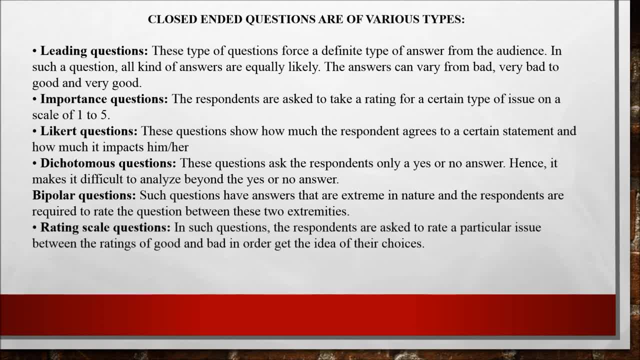 these two extremities and accordingly will let the questions go답ly throughout the shift difference. so is important to have specific collar lids in the envelope. so what this obviously says that it is not correct to raise only the khakra. it is i Schindler andussen's we call it. 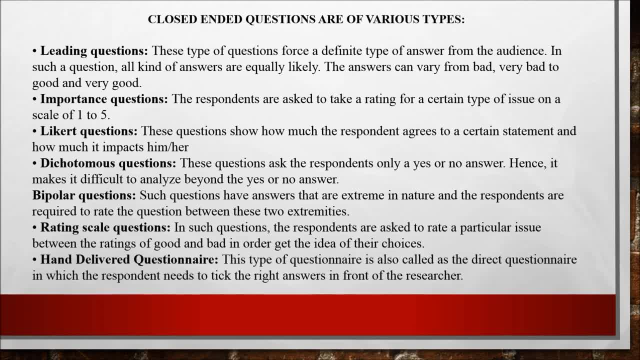 also said that the components visiting dining show waiting when the song of life fit rackett smallным deal in Karanta Alam isin. make a questionnaire for yourself right now. advantage of this method is that researcher has a close relationship with the respondent because you're directly going and involving. 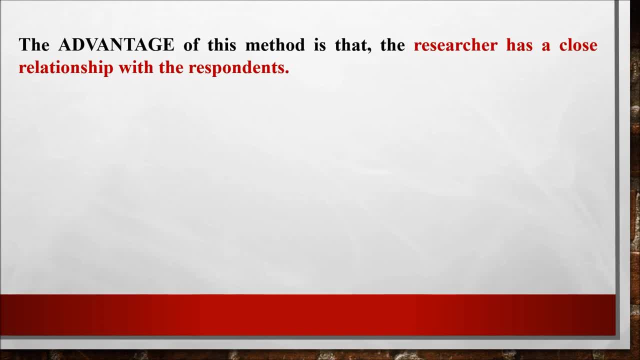 with the question answer, asking him certain things, learning his mannerism as well, so observing while he's answering. so this has a closer link with the respondent. then it accommodates tough questions. it means questionnaire may have so many tough questions that are explained by researcher to the respondent because respondent may not be aware. suppose i, if i say climate change and the 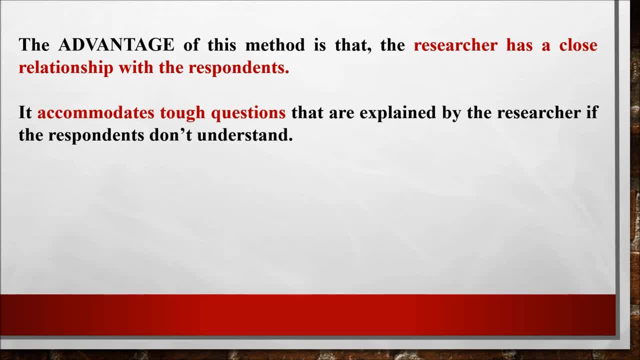 person is not well educated. he doesn't know what is a climate change, so what happens? it is a tough question for him, so in that case i explain him that what is a climate change phenomena? if he doesn't understand my language, then i have to translate it into his language for his understanding. 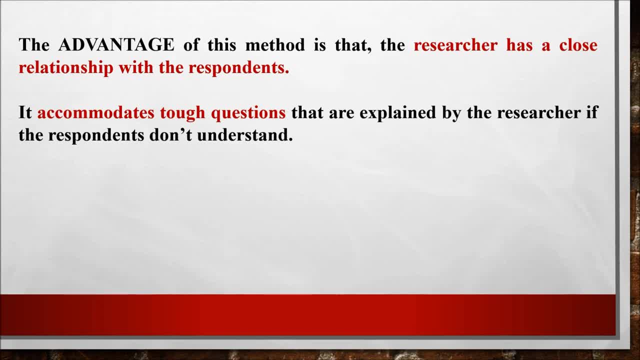 in simplicity. so this is what is there, that it can accommodate tough questions as well. in this method, reason or purpose behind the study of climate change problem is also described. so you tell the respondent that i am studying such and such event of phenomena or behavior. so that's why i am asking for such answers from you and disadvantage. 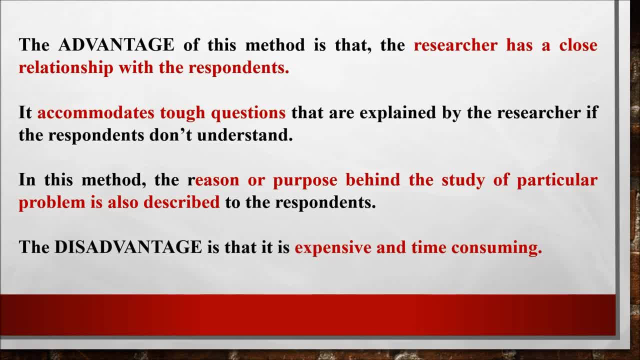 is that again it's time consuming and many times because going to the field is an expensive phenomena because of the again because it's time and also accessibility at many times. so what happens? a disadvantage becomes expensive and time consuming. part of the questionnaire method. now this is the most relevant. 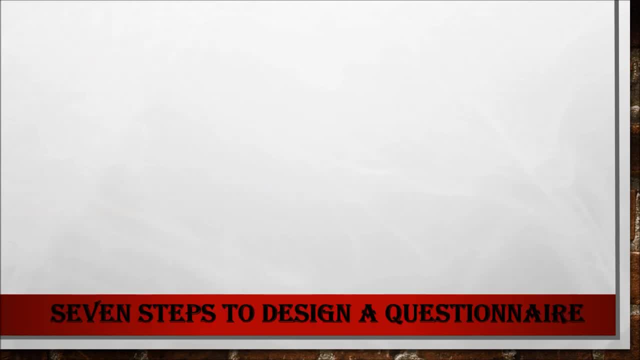 part of this session, i'll give you seven steps how to design a questionnaire. so remember these seven steps when you are making a questionnaire. what are those seven steps? the first is to identify the information required. so identification is the first step. so if i require information about loss, 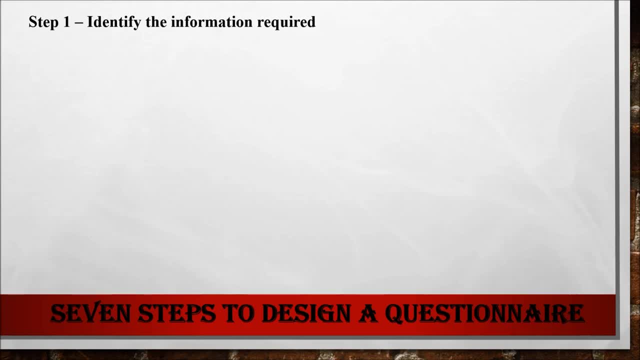 of water bodies due to climate change, suppose. so i clearly know that my question is about going to be about water bodies in a particular area, so i've identified my information required. it has to be involved with the water body. right then i'll give you seven steps: how to design a questionnaire. so 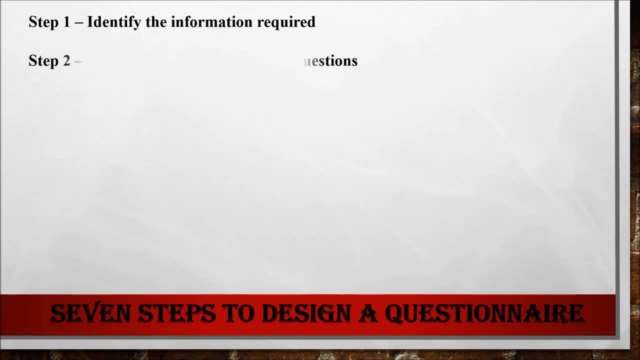 making a rough checklist of questions. so firstly, I make 20 questions or 30 questions of a rough checklist method, right, so these questions can be there. so roughly making a question, okay, then refine the construction of questions considering the respondents. now here comes the respondent part. if we know, 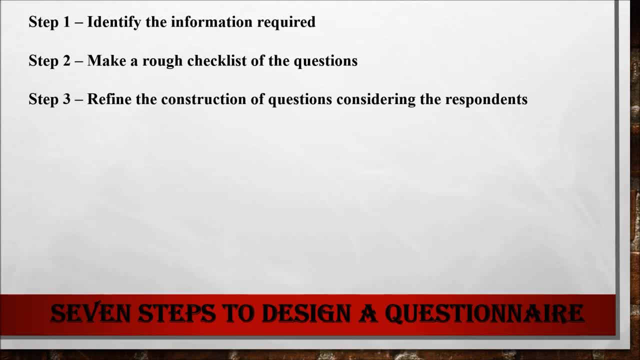 that the area where I am going to ask these questions. respondents are well educated, then it's a different set of questions, right? if they are not educated, if they're of too remote area, too rural background, then we have to do certain kind of simplification in the construction of questions. that is the 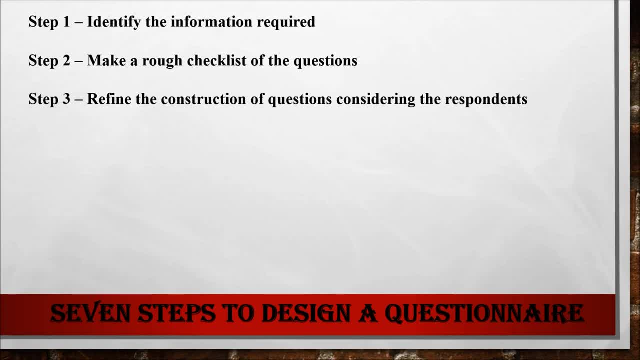 step three: now develop the response format. it means tables, tick marks. these are the fourth step. after this question structure is being there now, what kind of answers are thinking of getting back? so is it a tick mark based again? just now we discussed about several types of questions, so we need to decide on the 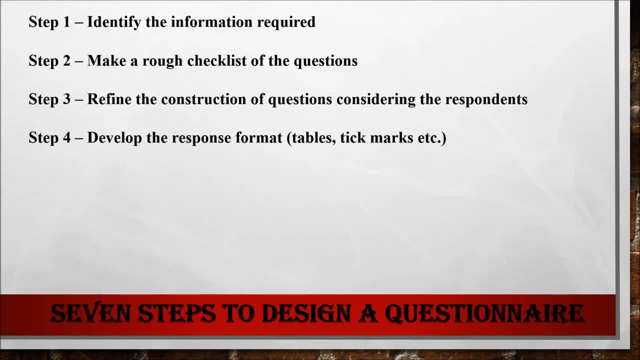 format of tables: tick marks, fill ups, rankings. so these are the fourth step, then fifth step, put the questions into an appropriate sequence. sequencing is very much important. randomness cannot be there. once you're asking his name and second question, you asking him his income. third, you are asking him about biodiversity. and fourth, 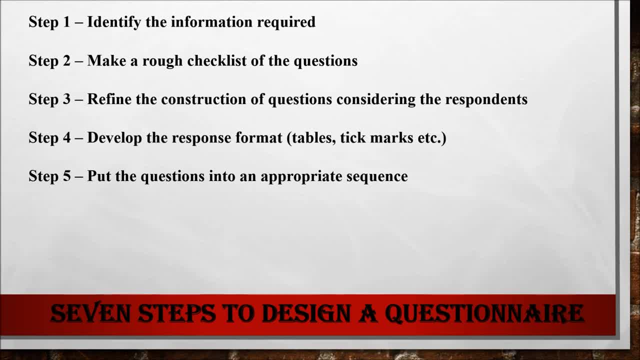 again you are coming back. is there a particular amenity in your house? so this is non sequential, right. so personal questions, that is, about the person, his family, then income, then assets, then about the crux of the matter that you're looking to. so your objective based questions and 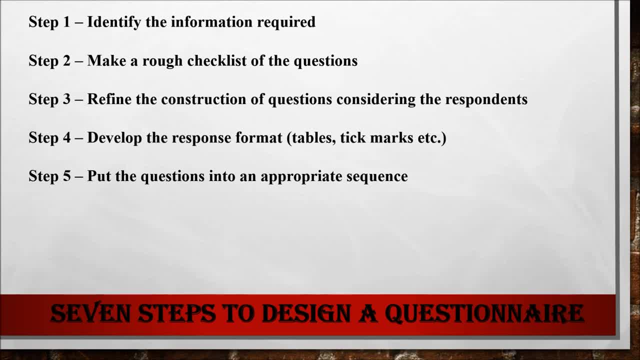 then the last summary. so this has to be a sequence in the appropriate way: right the questionnaire. so that is fifth part, and sixth is to finalize the layout of the question. so layout finalization is the sixth part and then seventh is pre-test and revise the questionnaire. remember questionnaire normally people 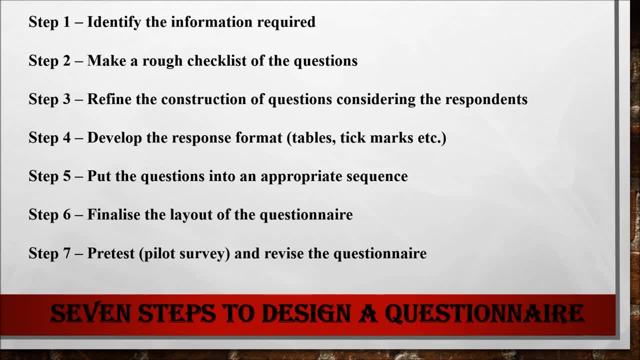 don't do this seventh part. they finalize it in the sixth step and just go to the field. remember, always spend a day or two in the field just to finalize and revise your questionnaire on the basis of a pilot survey. just take those questionnaires to people and ask questions and see the difficulty that. 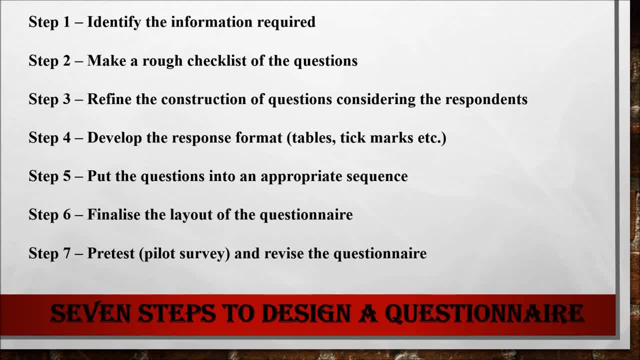 you're facing and then revise it and then again go the next day. this is the way it should work, okay? so if you don't understand, then what happens? there is a problem when you get these responses back and then you start tabulating them, so in that stage there is a problem. so remember these. 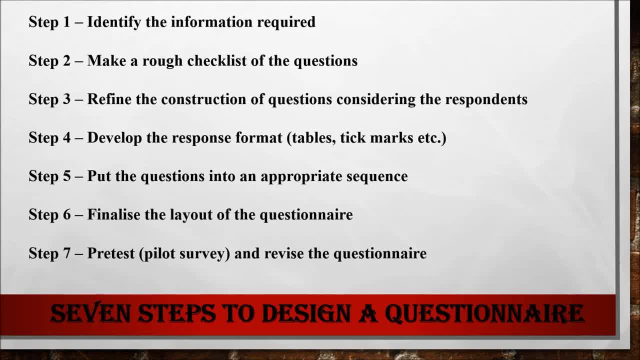 seven steps. these are the seven key method of designing a questionnaire. alright, so I hope you'll have this method very much clear in your head. is seven important points. and whenever you go for a fieldwork, first they spend time in your field doing a pilot survey. do not do the final survey on the first day. 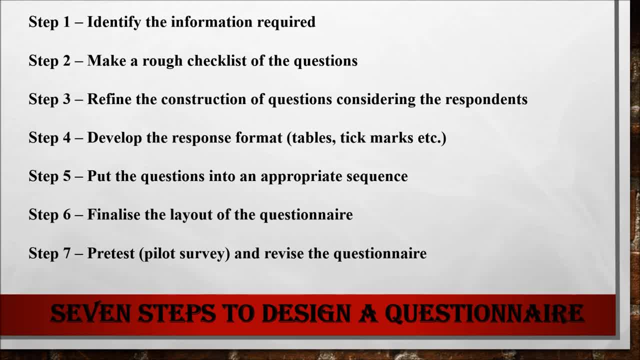 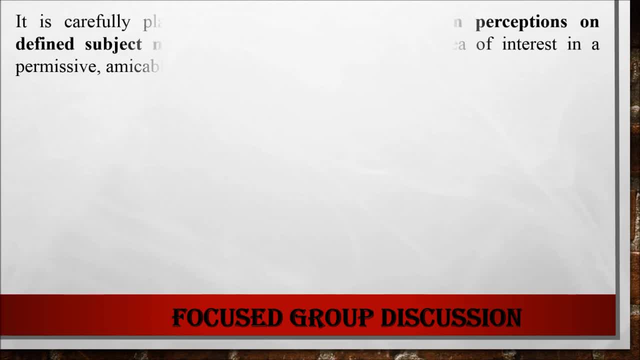 that's very much important. then focus: group discussion. so this is the third method of today that we're going to discuss, as this word is group discussion, so it is carefully designed and planned way of asking questions to obtain perceptions on a defined subject matter by the entire group in the 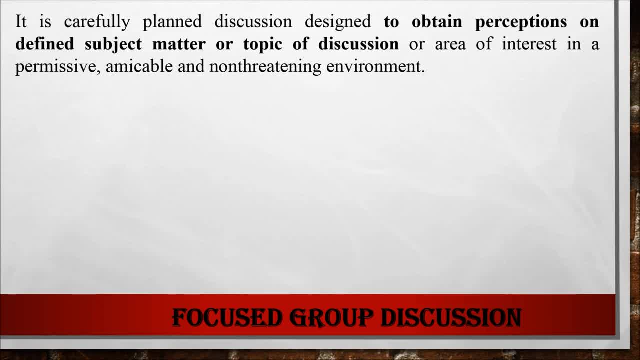 area, for example, if i say climate change now, i'll bring people from different parts of the society and make them sit together across the gender. you know male, female and other genders, so all sit together. so i have i'll compose a group and then i'll give them topic of discussion and ask them. 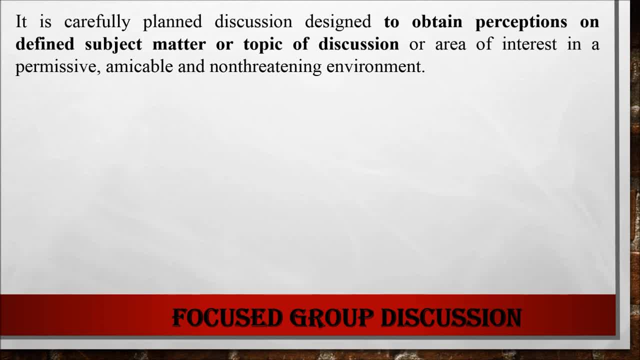 what is your opinion about it? what's your perception about it? so this will start a discussion on that right. so it is conducted with approximately five to ten people, not more than that, so a healthy discussion can take place. okay, and you understand, and for this we need a moderator over this. the. 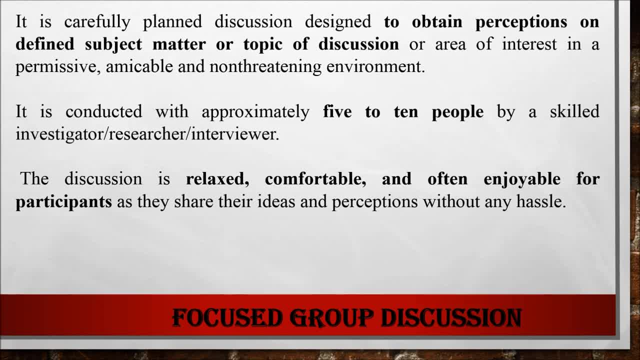 moderator can be researcher himself or a senior person of the community, who you can appoint as a moderator, all right, that's important. the discussion is relaxed, comfortable and often enjoyable for participants because they share their ideas openly, freely, right, without any hassle, because they're talking amongst themselves, amongst their community and what you 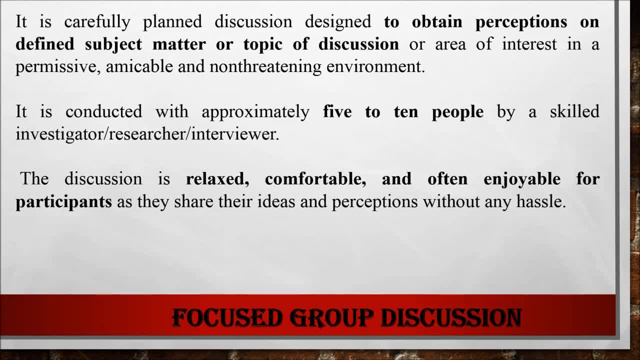 are doing as a researcher. you're just noting down their viewpoints. that's important. while they're talking, you're just noting down, right. then group members influence each other. so by responding to ideas and comments in their discussion, it's important that they must respond to each other. so advantage of focus group discussion: it's a important phenomena in which 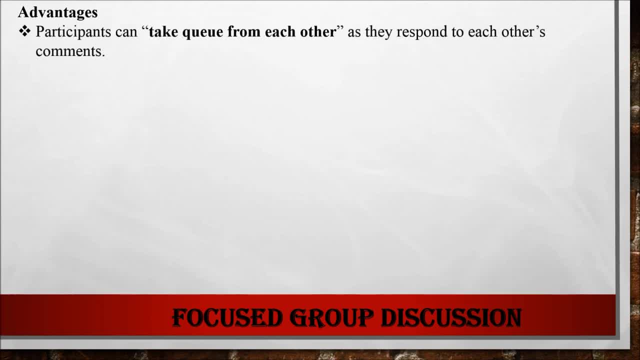 these people take cue from each other. suppose i said something and then somebody looked at me and it took a cue from what i said and then he has something to say. so this is one important point. they may agree or disagree. that inside you to see it, isn't it so? disadvantages this difficulty management, because many times 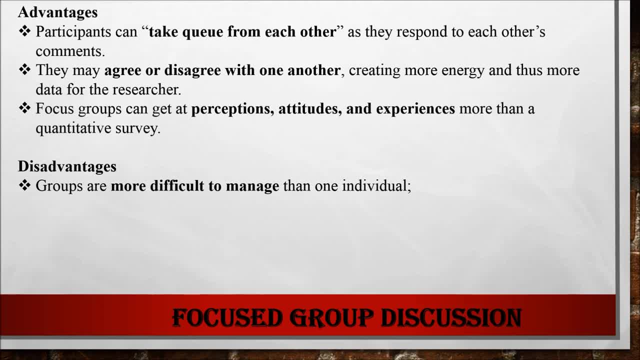 individuals in a group are difficult, they may not be on the same page, conflicts may be her powers struggles to be there between them. but I said, and then he has something to say, so this is one important point. he may agree or disagree. that gives a variety in the answer. then again, perceptions, attitude, experiences, these are the things that add on. so this is an addition to what can not get just in a questionnaire, isn't it so? disadvantages: it is difficult, management, because many times individuals in a group are difficult to manage, they may not be on the same page. so the conflicts may be there, power struggles maybe between them. there a little bit higher disorder, or instead be in British, I don't know, but it might be an sensory lives, because he ispping confidence with a group, whereas language is a history. so there grilled English and that with 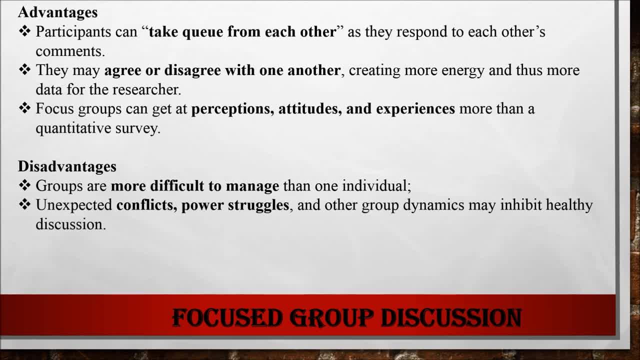 difficult and shy. people may be also intimidated when you are asking certain questions or somebody is shouting in a group and somebody is like, okay, i won't answer or i won't say anything, so this can be a problem. so these are the disadvantages, so we must take care of advantage as well as. 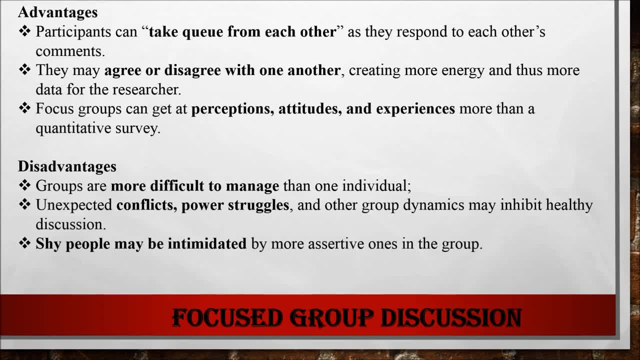 disadvantage of every technique that we are learning, like focus group discussion as well. right, so moderators and facilitators, whosoever, have to be really skilled to handle this focus group discussion. it's not an easy method to get data, so remember if we are using focus group. 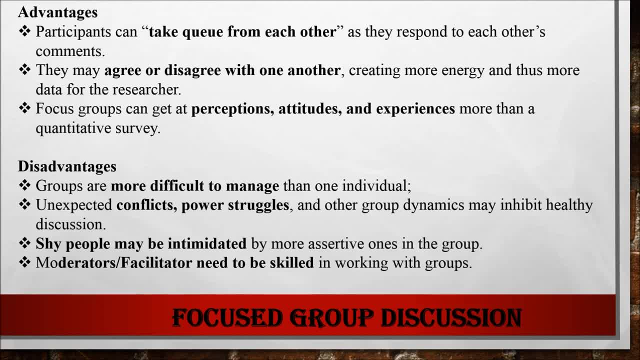 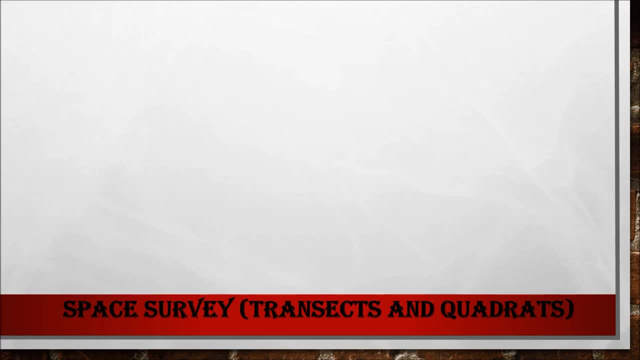 discussion in a particular region or area, we must have a skilled moderator with us, otherwise it will be a disadvantage for us. right now, space survey- the fourth and the last part of the surveys that we conduct in the field. this has two types: transects and quadrants. now let's look at this. 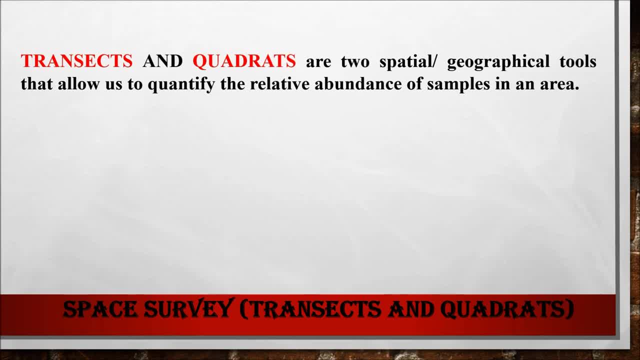 so transects and quadrants are two spatial geographical tools. okay, that allow to quantify the relative error of the data and the data is then used to quantify the error of the data. the problem with the transects is that both of themics can be done in the regular intervals. 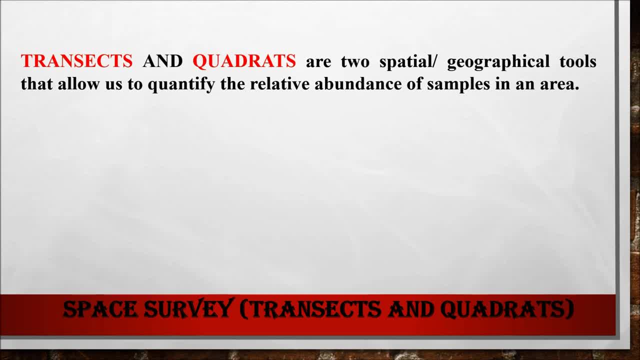 thank you for watching. we will see you in the next class. Suppose: if I draw a line, that line can be a length of a road from point A to point B, And then it is easy for us in the field to order, select samples, For example every 5 steps on the road or every 20 steps on the road, isn't it? 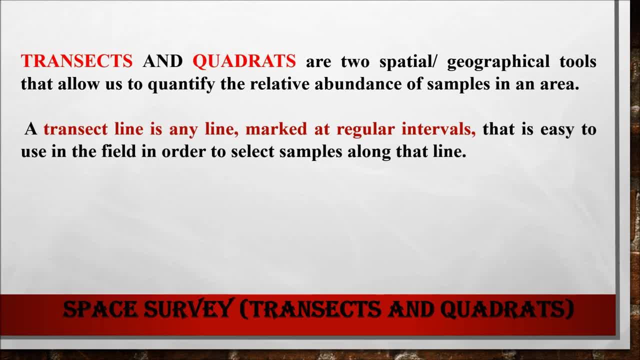 Or along the canal, So any line feature. if I opt in So that case, that line feature will be our transect line because it is along a canal, along a road right. So, for example, selecting a sample village along a river in order to check the impacts of flood. 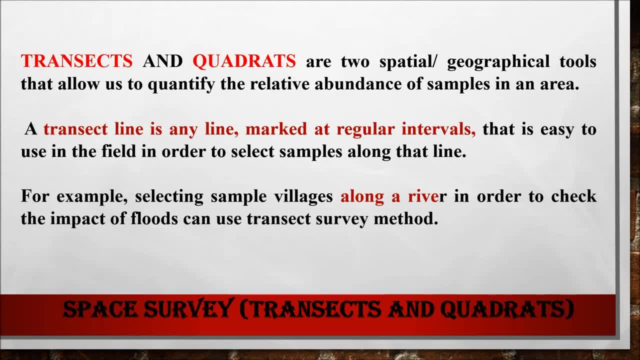 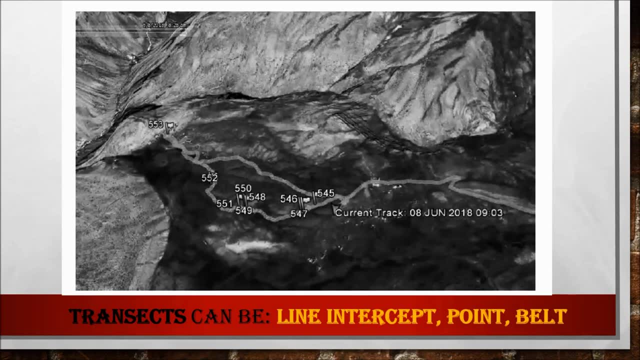 So what can happen? If we decide upon, then we can select that transect line and, along that transect, whichever settlement keeps coming, we can keep asking questions, right. So that's how transect is done. For example, if you see this image, this is an image from a mountain area where, using GPS, the transect line has been defined. 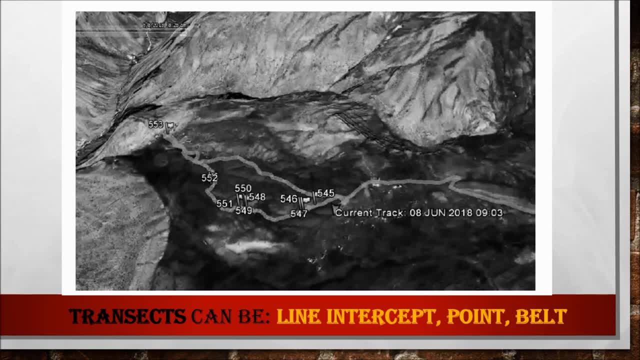 And those are the places where the person stopped and asked questions or collected samples. So first you decided your area, Your line of intercept- that can be a particular line, point and belt- and then you collect the data on that particular line, along the entire line. 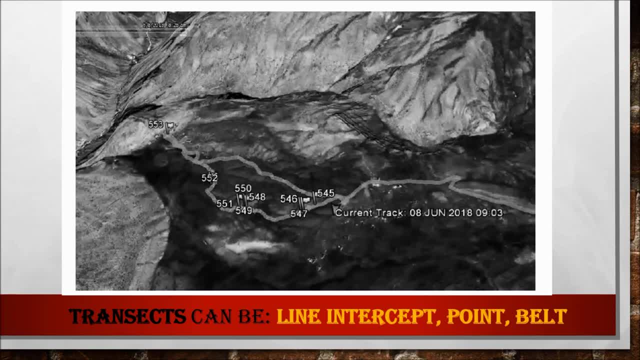 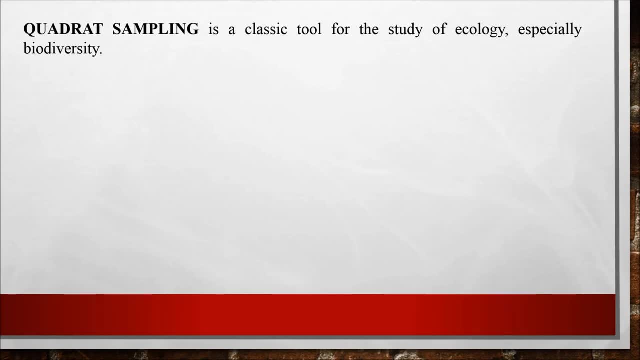 So that is how a transect survey is done in the field. Then quadrat sampling is a classical tool for ecology, especially for biodiversity. So what happens? It has a series of squares. That's why quadrat, quadratic equation, if you remember. 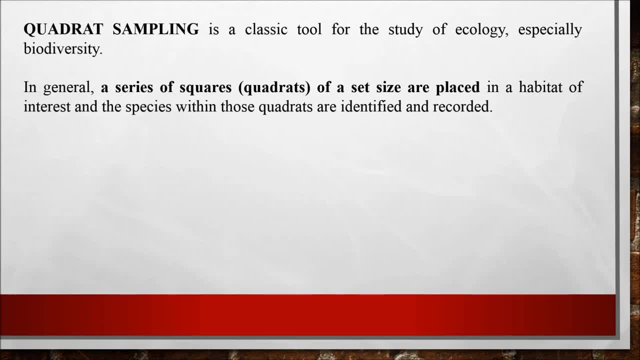 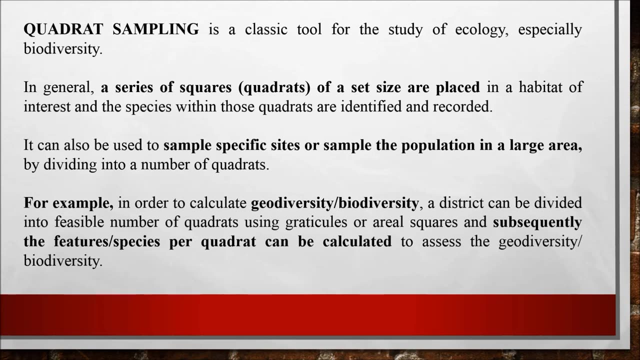 So quadrat is the name of a set size, So it is basically a square. And now what we do? We divide the area into specific squares or a sample site, into particular population area And, for example, diversity studies, biodiversity, geodiversity. such studies can be mapped on this line of surveying, that is, quadrat sampling.